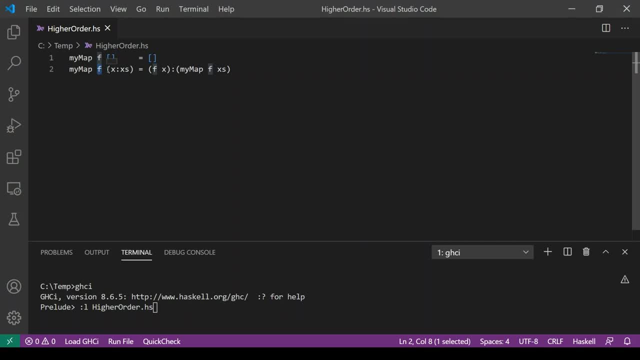 which is a list, and the returned result will be a list with all the results of applying the function f. I can interact with this code and I can see that the function f is a function of f and use several existing Haskell functions, such as absoluteValue And if I apply MyMap. 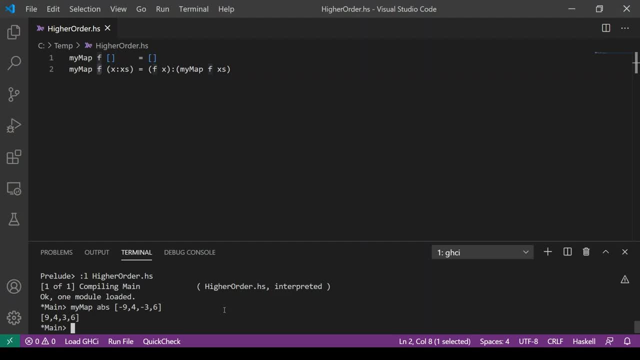 to that list, I get all positive results. I can also apply something like multiplication times two, and the values from the list will be plugged in as the first parameter of the multiplication, And so when I apply this, I get the result of multiplying each of these. 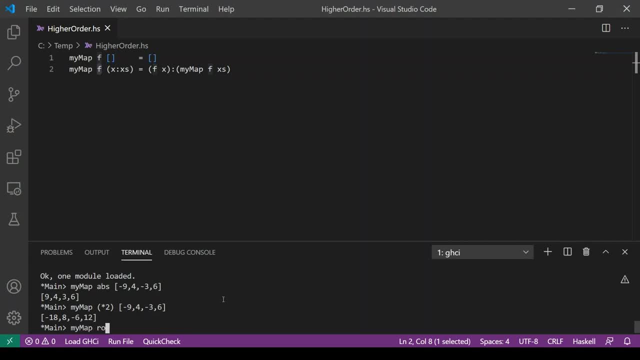 values by two. I can also use the round function to round a list of values that have decimal components. So this definition is fairly simple and, strictly speaking, the occurrence of f here in this case could be changed into an underscore, because I'm not going to have to. 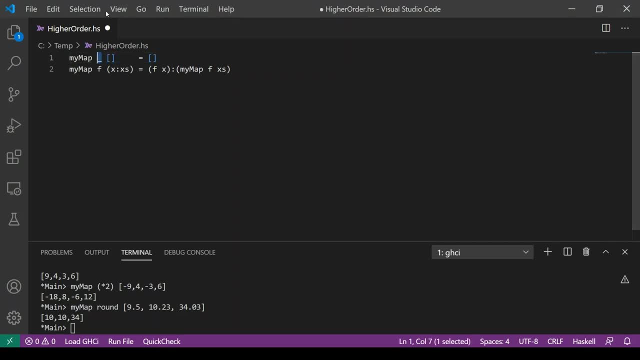 do anything about this, because when the list is empty, it doesn't even matter what the function is. Now, interestingly, Haskell's type inference engine means you don't have to explicitly declare your types, But you can ask what the type of any function is. 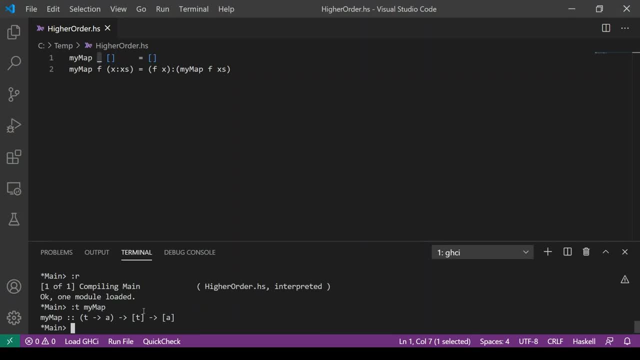 and Haskell will tell you, And what we're shown is that the MyMap function takes as its first parameter a function from types t to types a, and its second parameter is a list of elements of type t and its output is a list of things of type a, t and a are. 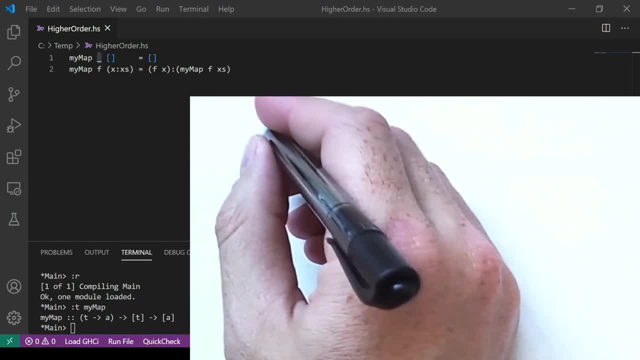 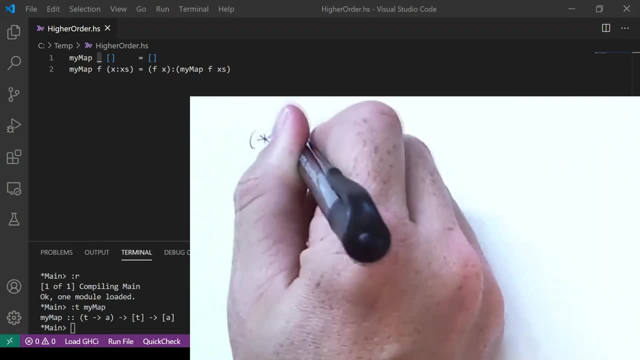 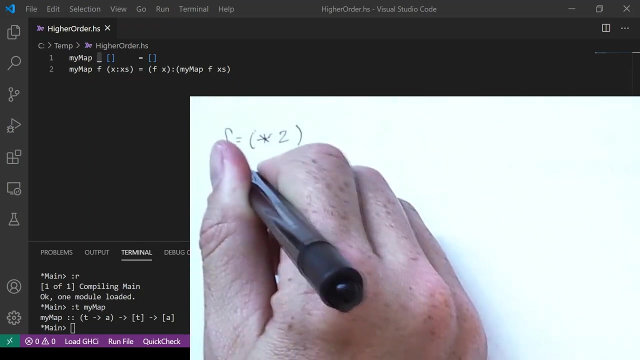 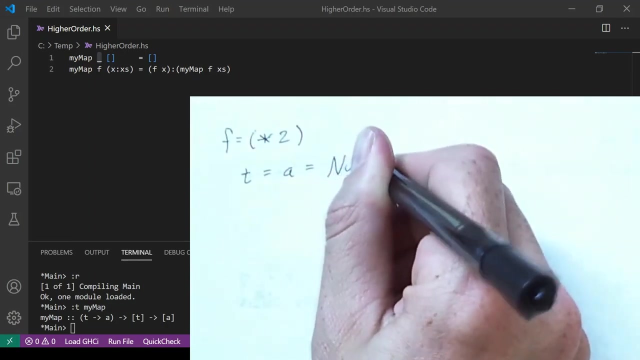 type variables that get mapped to specific types when you apply the MyMap function. So when I'm using multiply by two as my function, f, well, in that case both t and a are going to be arbitrary numeric types, because the function for multiplying by two is of type. 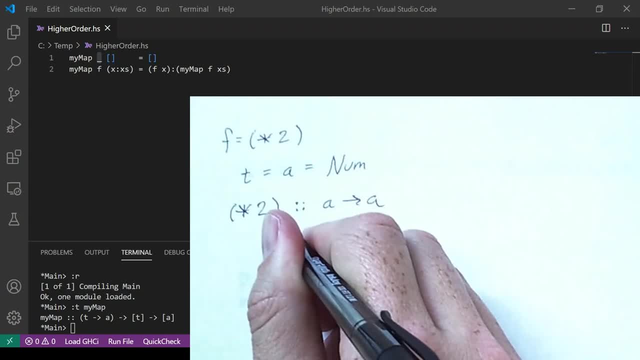 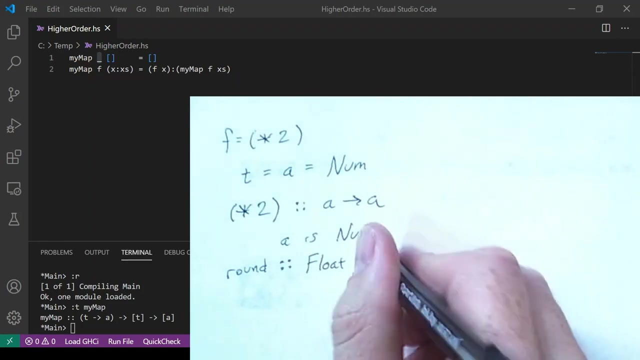 a to a, where a is numeric. If I'm using round, well, this is a function from a floating point numeric. If I'm using round, well, this is a function from a floating point value to an integer value, which means that float would be the t. 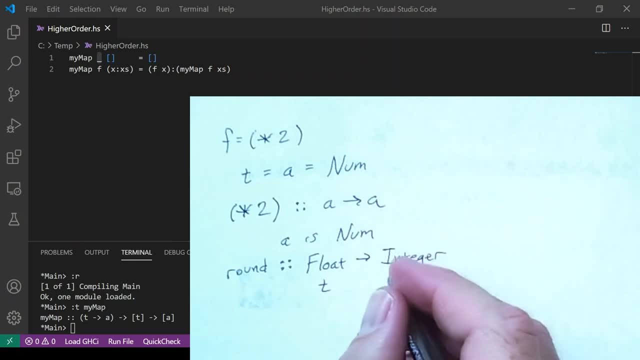 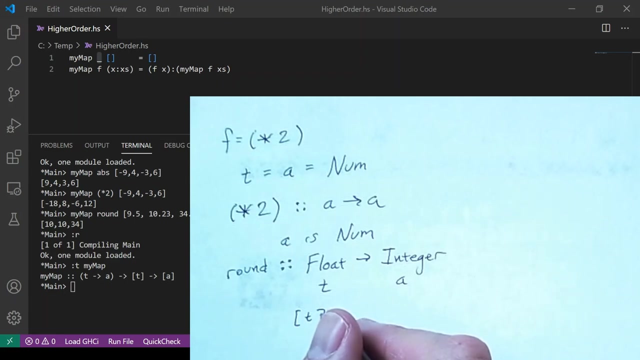 and a would be the integer in the type signature for my map. That's why the input is a list of type t or, in the example I gave a list of floating point values and the output is a list of integer values. Basically, what map does? 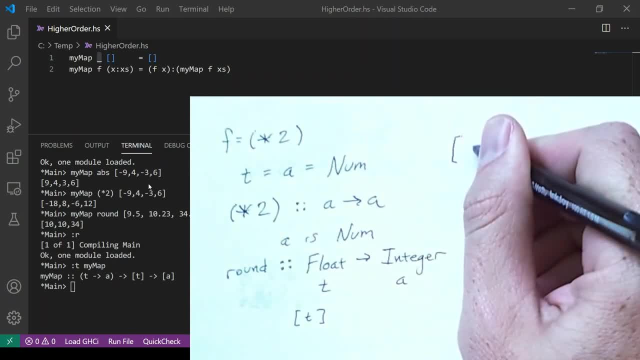 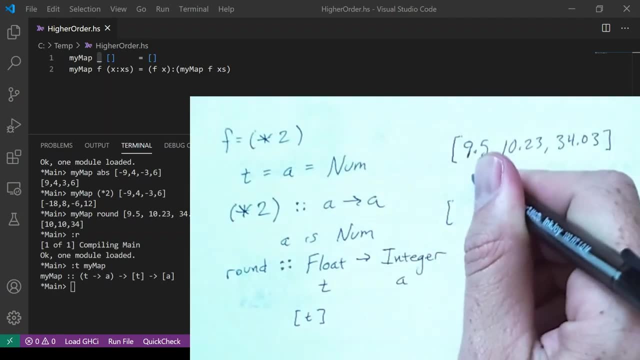 is. it takes a list of one thing- let's say, in our example we're using the floating point values- and, without changing that list at all, it creates a new list via application of the round function. that has all the results. In fact, this type of operation is so useful. 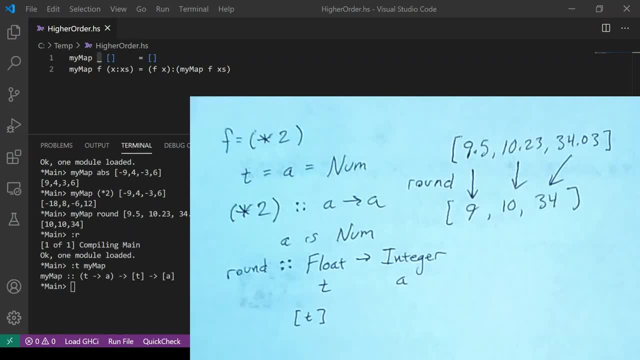 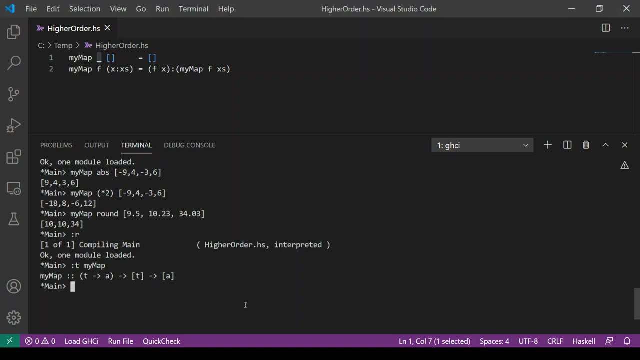 that Haskell actually has a built-in function for it, simply called map, And map behaves exactly the same way as the my map function that I defined for you. I can use map with multiplying by 2, I can map the round function and if I check the type of map, 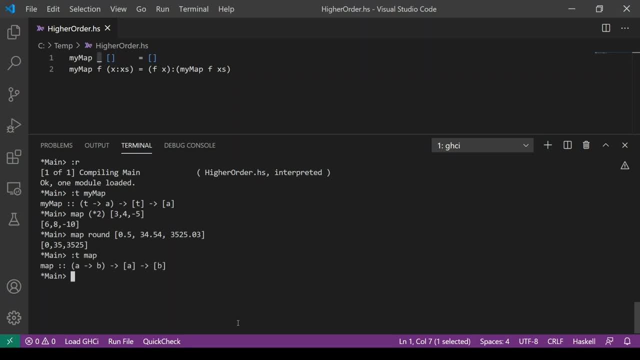 you'll see that it's the same, although the specific names of the type variables happen to arbitrarily be different. Once you're used to the existence of these higher-order functions, it makes it very easy to define other functions in a simpler way. For example, here is how you would define: 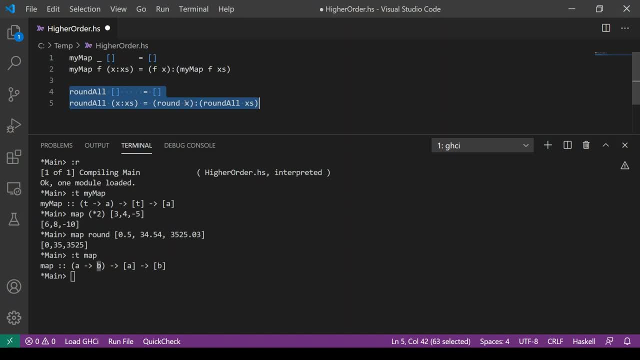 a function that rounds all the floating point values in a list without using map. You would have a case for the empty list that leads to an empty list, and otherwise you'd round the first element of the list and then recursively call roundAll on the tail of the list. This function works fine. 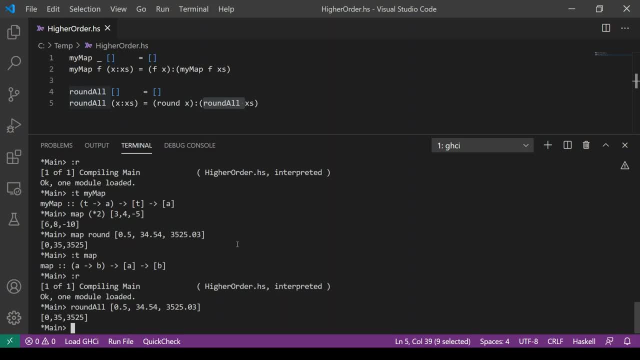 and gives us the same result. but I could simply define it in terms of map like this: Here the HO stands for higher order, and notice that I don't even have to specify the parameters. I could specify that there is a list xs and that I'm going to map the round function to that list xs. 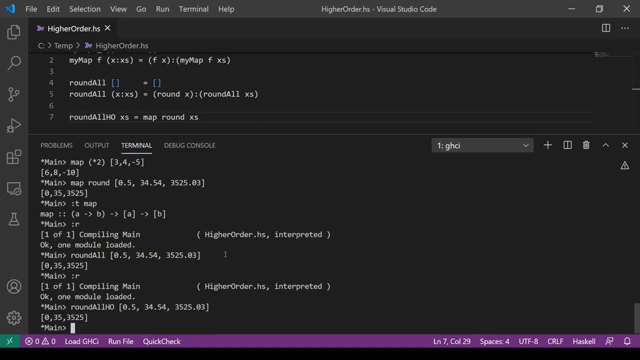 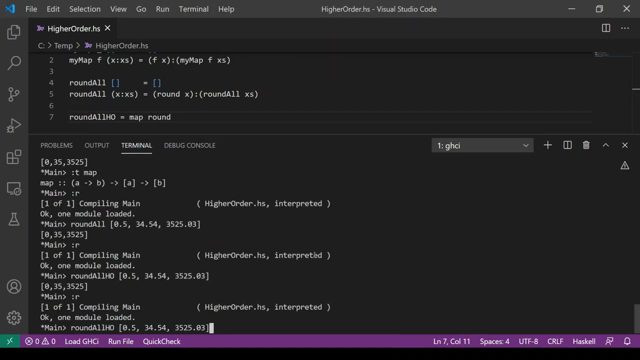 And if I run that code, it will work. But when you have the exact same parameter at the end of both the left-hand side and the right-hand side of a Haskell definition, you can simply erase it and get the same result. You can also return functions. 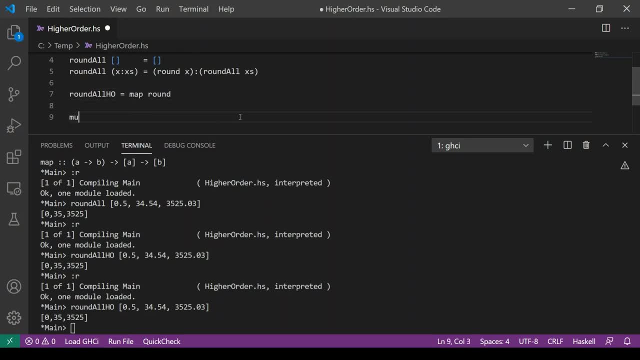 from other functions, and here is a simple example of that. This multiplier function will return a function that multiplies one value by whatever that one parameter was. So, in other words, multiplier x returns a function that will multiply any other value by x. 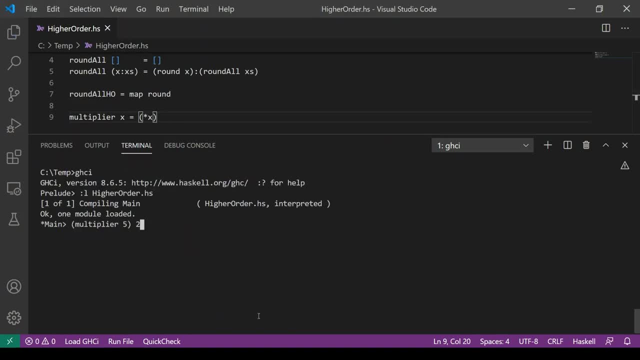 So I could call multiply with a value 5 to create a function and then apply that function to the parameter 2 to get the value 10.. I could also send my multiplier results to the map function. So I have a function that will multiply values by 10,. 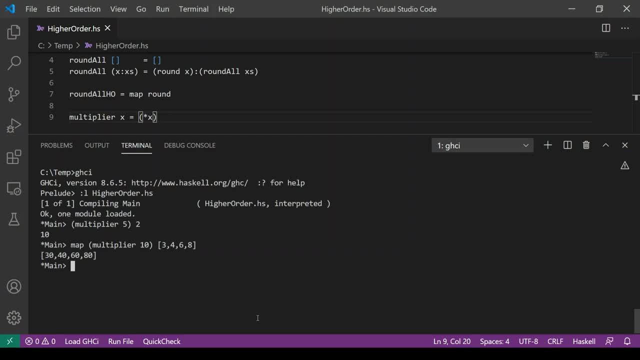 and then I send that function as a parameter to map to multiply all the values in a list by 10.. Another common pattern we see is that of taking a list and repeatedly applying an element to pairs of elements in the list, such as when computing a sum. 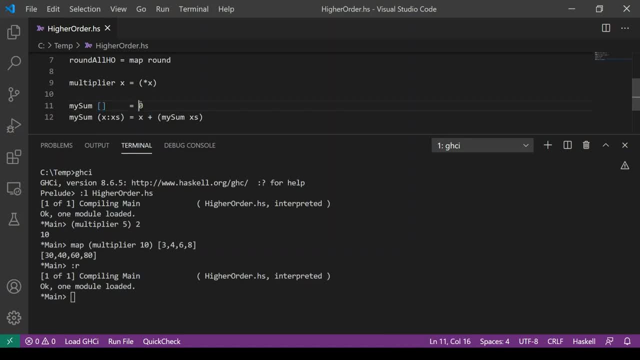 If we're getting the sum of elements in an empty list, the result is 0. Otherwise we take the first element and add it to the result of summing the rest. So I could call my sum on the list 1,, 2,, 3.. 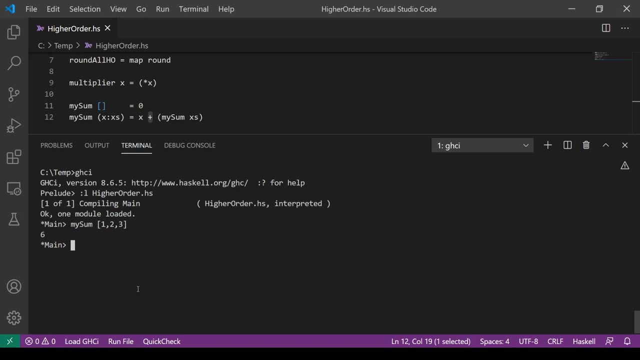 That's 1 plus 2 plus 3 plus 0. In fact this is equivalent to computing 1 plus parentheses 2 plus parentheses 3 plus 0. Close, close, close And I get that result. Notice how the parentheses bunch up more on the right-hand side over here. 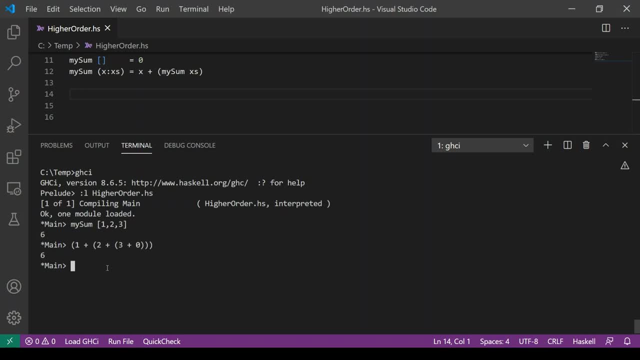 This kind of operation is an example of something called folding, And because the parentheses are bunching up on the right, it is specifically a fold on the right side. In other words, there's a function in Haskell called foldR And it can accept another function. 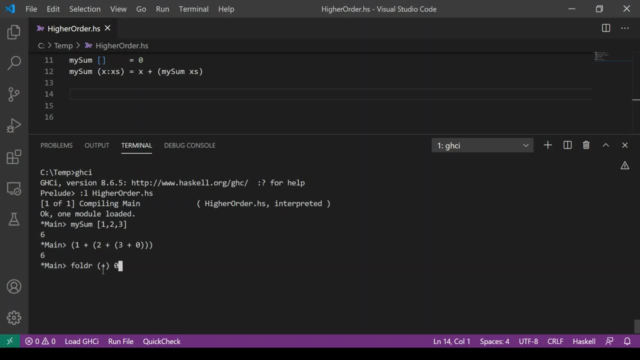 It can accept a function as a parameter and a base element, And if I send it the list 1,, 2,, 3, we'll see that we get the same result here. So foldR takes this plus operation, sticks it between elements of this list. 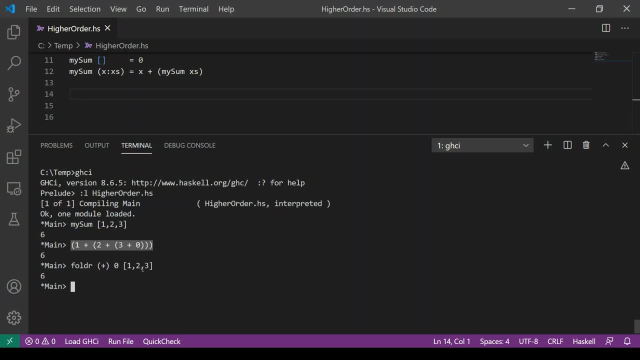 separated with parentheses in the way we see there, with 0 as the rightmost element in the innermost parentheses. I can actually define a function this way. This is mySumHigherOrder, And here I've explicitly declared the type of it, because the foldR function can sometimes be picky. 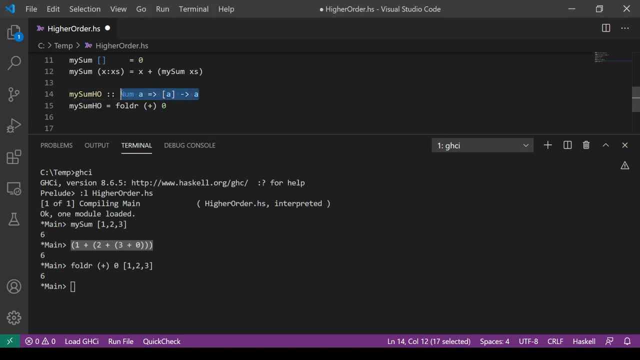 And Haskell might complain if I don't explicitly indicate that this is a function that takes a list of numbers and produces a single number. But that is the same definition that you saw me use in the code right there And if I reload it I can call mySumHigherOrder. 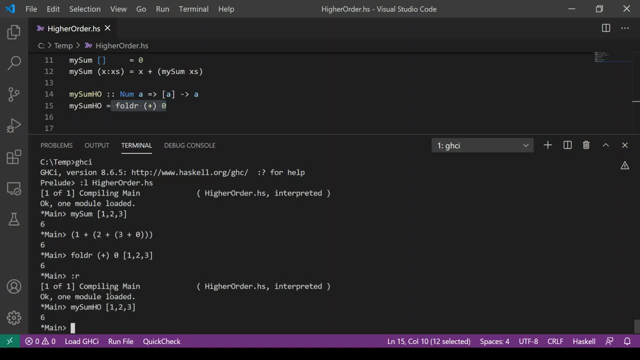 on that list and get the same output. Now, the type of the fold function is very complicated. It takes a function of two elements that returns a third, And notice that the inputs don't have to be the same type. In the case of addition, both my inputs were numbers of the same type. 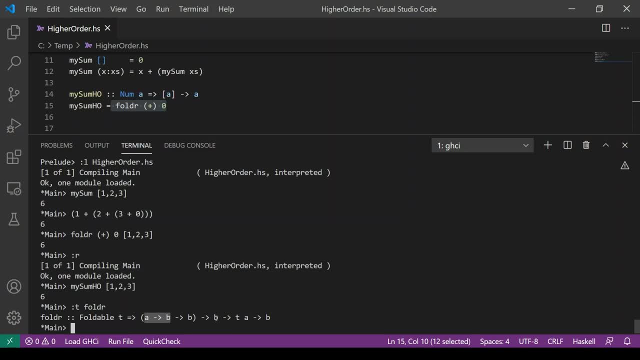 But folding is more flexible than that. b is the base element. In our example it's 0.. And ta is indicating that you can fold across things beside lists, And so we happen to be folding across a list, And so what we have is a list of numbers. 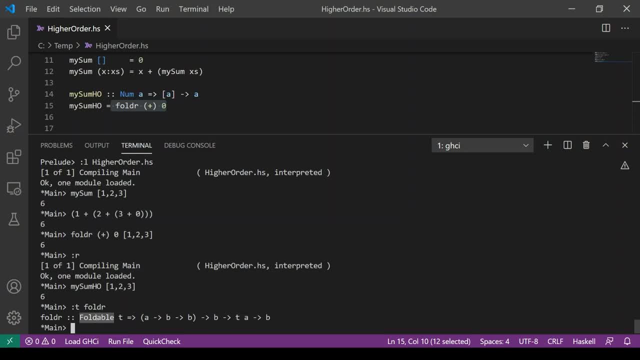 But there are other data structures we could fold across that are designated by this foldable class, And then, finally, we have the result that we get at the end. There is a corresponding fold function called foldL for foldLeft, And if I were to apply foldL to the same values, 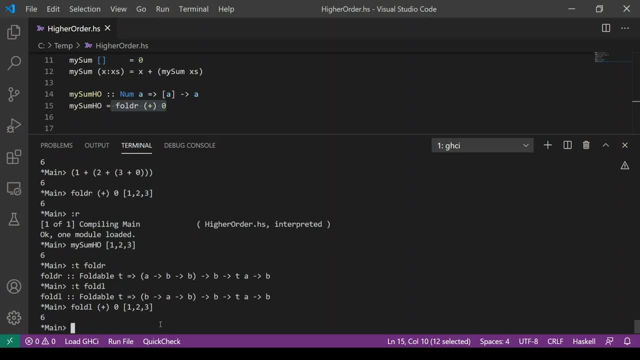 I would get the result. But that's only because with addition it doesn't matter what order I compute. the result in FoldL is essentially computing 0 plus 1 plus 2 plus 3.. So it's grouping the parentheses in a different order. 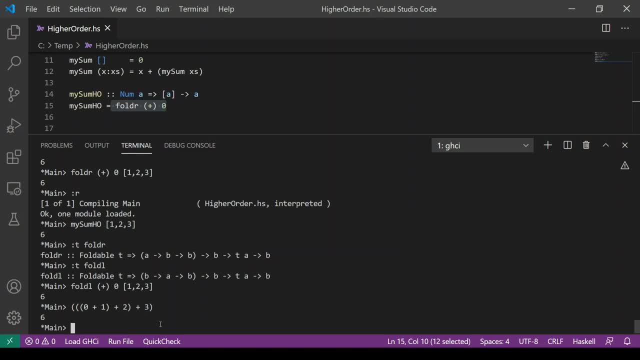 Which works fine for addition, but if you do this with subtraction, you get a different result than if you use foldR, And I'll let you work out the details of that on your own, Though understanding how these fold functions work can be difficult. 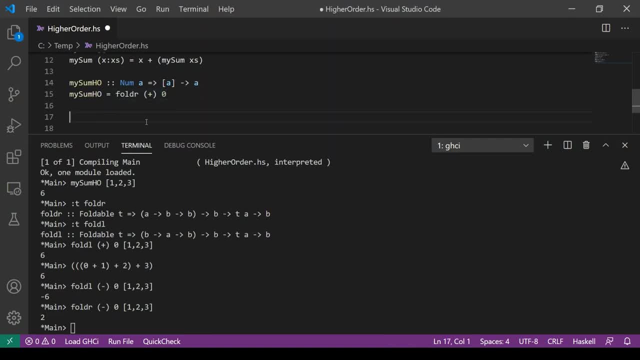 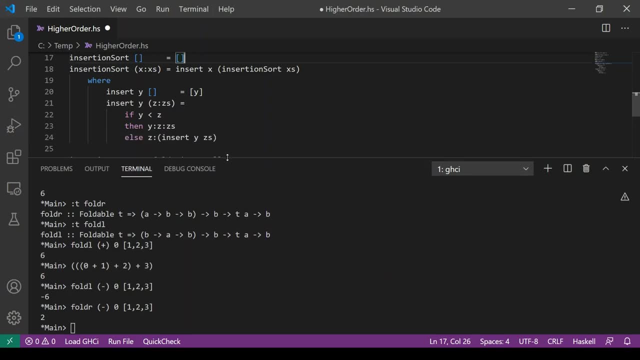 it is a very powerful way of defining many complex operations. In the previous video, I defined insertion sort as shown here. However, we can actually think of insertion sort as simply a fold operation on this insert function, So we have both this version of insertion sort. 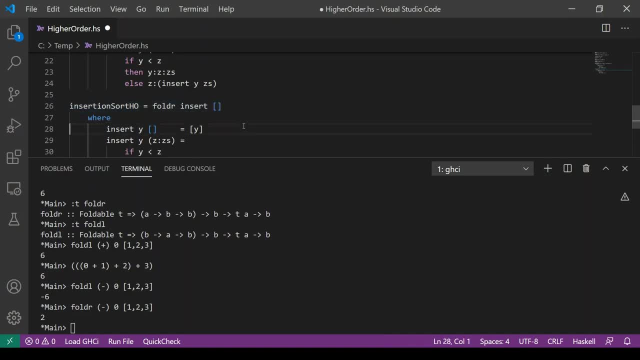 as well as a higher order version of insertion sort. The insert helper function is defined the same way in both instances, And I can make this more explicit by removing it from the WHERE clause and simply letting it be its own top level function. So clearly, both versions of this code are using the same insert function. 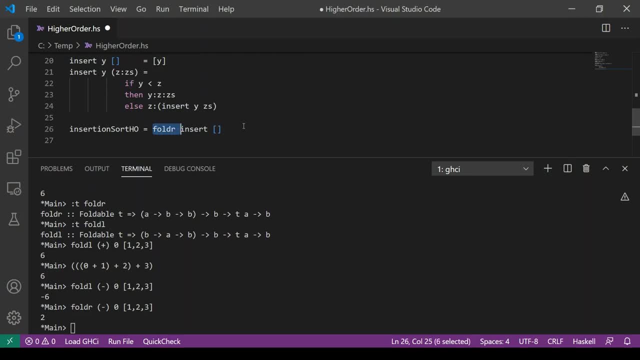 But the higher order version simply has to fold the insert function across an empty list. Once again, we will need to provide a type signature to make it easy for Haskell to interpret what is happening in this function. So what this type signature shows is that the elements of our input list have to be. 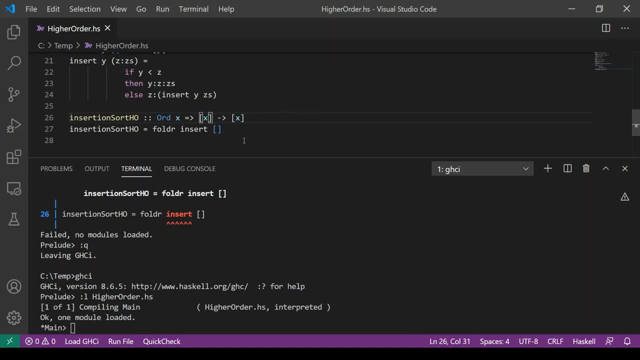 orderable, There has to be a way of comparing them using less than, etc. So we take one list of orderable things and output a new list, And of course we know that it should be the same elements, but in sorted order. 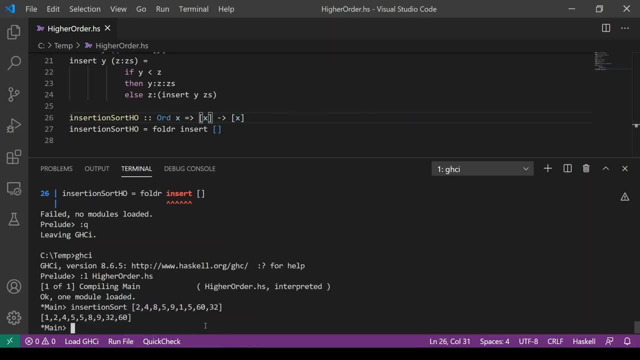 So the standard insertion sort did not use the fold function And it gives us this result. But if I do the higher order version, I get the same result. Haskell has many other useful built-in higher order functions you can use, And as you write more and more recursive functions, you tend to find that most of what you would 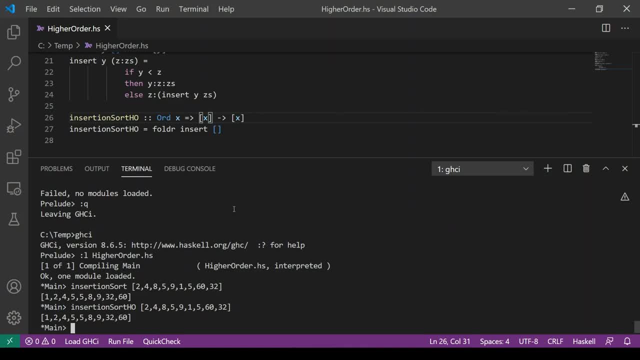 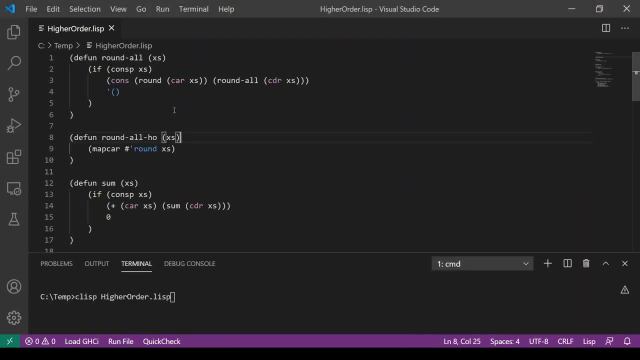 ever want to do can generally be encapsulated by one or more pre-existing higher order functions, And once you can see these patterns, it allows you to eliminate a lot of repetition in your coding. Common Lisp also has a large assortment of higher order functions. 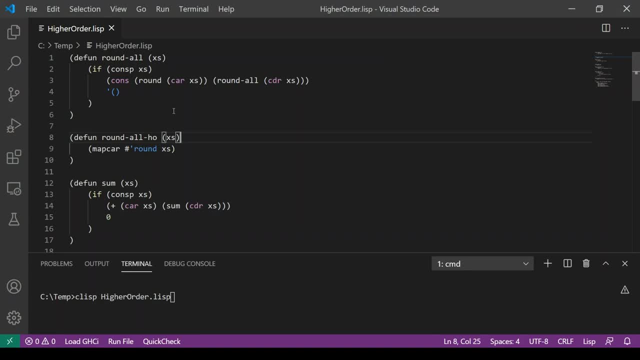 And what I've done here is define several of the functions we saw in the Haskell code using Lisp in both standard recursive style and in higher order function style. So here is a function for rounding all the elements in a list using straightforward recursion. We check if the list is a cons. 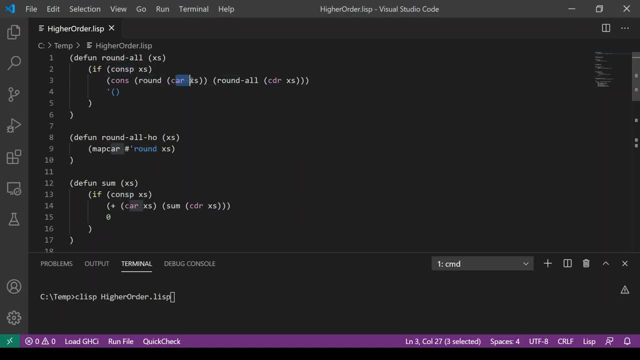 If it is, And we cons the result of rounding the car of the list to the result of rounding all of the ctr elements. Otherwise we return an empty list. This matches a map pattern, And in Lisp there are several different map functions, And the one that's most analogous to Haskell's map function is called mapCar. 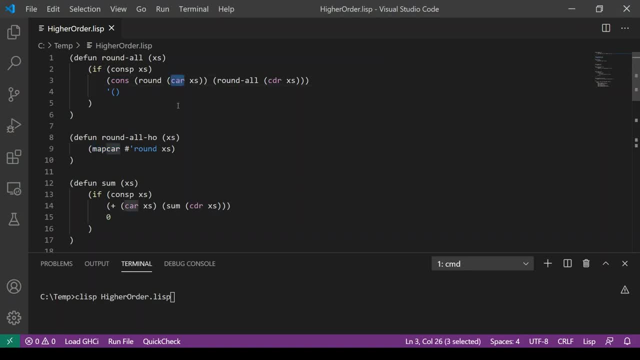 The idea is that we keep taking the car of the list, as shown here, apply a function to it And put all the elements together in one Lisp result. Notice that the name of the function has both a single quote indicating that it is a symbol. 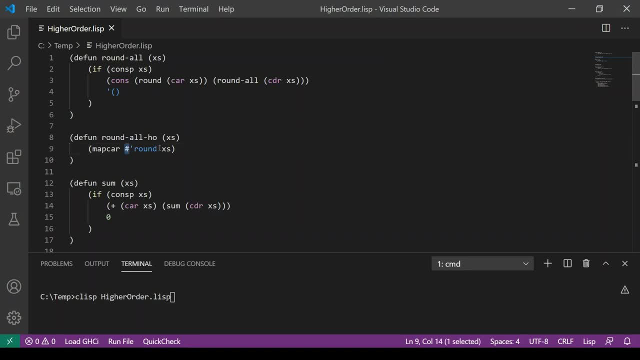 and a pound sign or hashtag that makes it clear that it is a function. We can also compute a sum in Common Lisp, both recursively, as shown here, and using a higher order function that is similar to folding Mhm. behavior of the reduce function is actually somewhat similar to Haskell's. 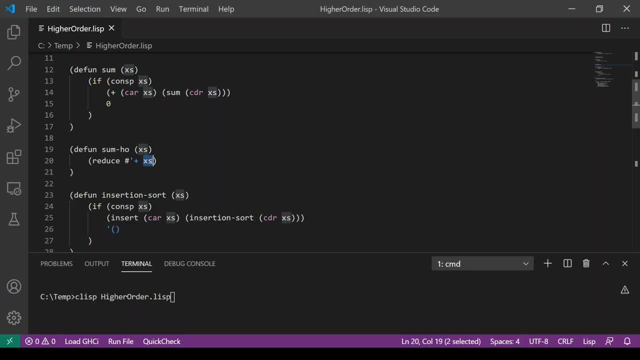 fold left- function. Here I have my list input and my function symbol plus has the single quote and then the pound sign to indicate that it's a function. I can also define insertion sort using reduce. First we have the recursive version of insertion sort, which is the same as what we saw in the previous video, and then 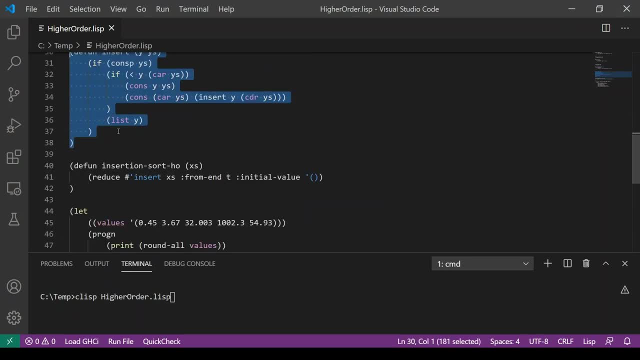 here is the insert helper function, and the higher order version of insertion sort will use the insert function, but we have some extra stipulations on how it is used. We specifically indicate that there is an initial value, which is the empty list, and notice that we didn't have to explicitly say that zero was the 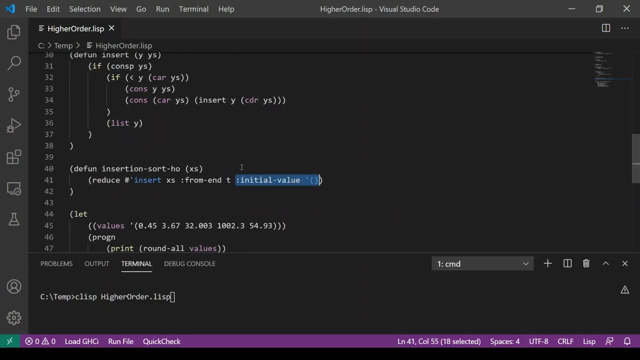 initial value. As soon as we press the X button, we can see that the value of the initial value when using reduce for sum- And we also want to say that we're going to start from the end- This basically makes the reduce function fold from the 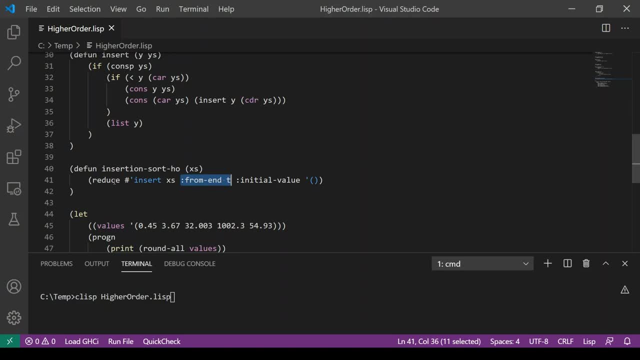 right as opposed to folding from the left. So what you can see here is that common Lisp's reduce function is a bit more powerful because it can do what Haskell's foldR function does and what its foldL function does. In fact, Haskell has two additional folding functions which have slightly different type. 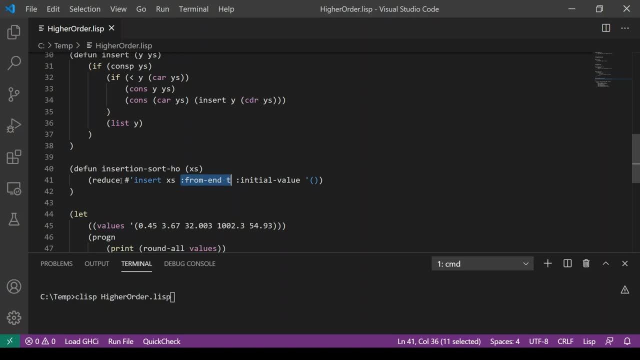 signatures And in common Lisp. all of that would be handled by this one reduce function. But to make it behave properly sometimes requires unusually defined parameters like these. This colon syntax indicates a named optional parameter, So the default value of from end would be false, for example. But I'm saying I want. 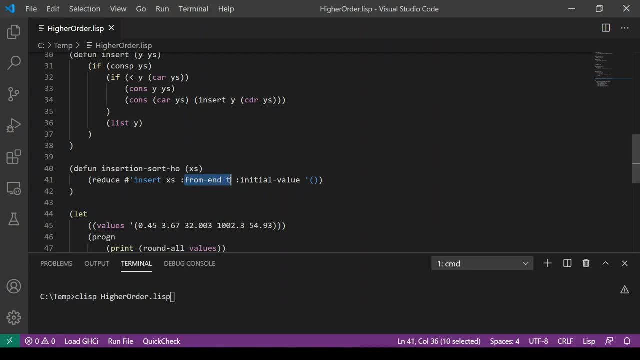 to use the from end as the default value. So I'm going to use the from end as the default value. So I'm going to use t for true to make it be folding right as opposed to from the left. Regardless, there's a bit of code here at the bottom. 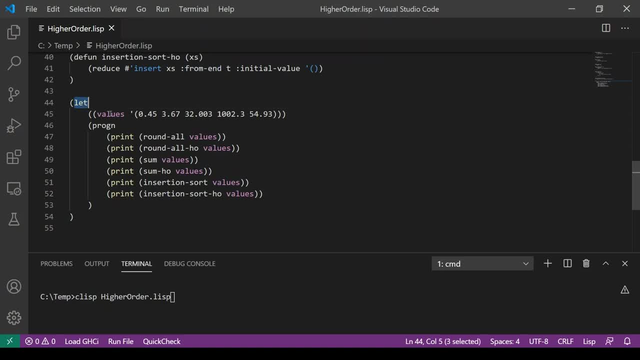 that tests this all out. We let the variable values take on this hard-coded list of values And I both round all those values using the recursive approach and the higher order approach. I get the sum using the recursive approach and the higher order approach And I sort all those values using the. 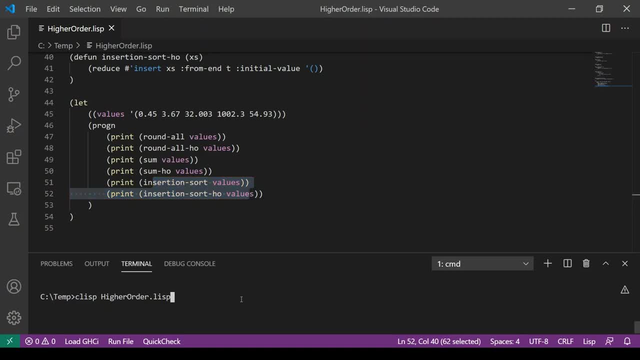 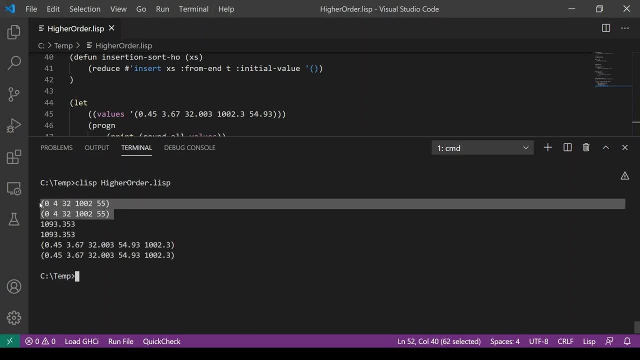 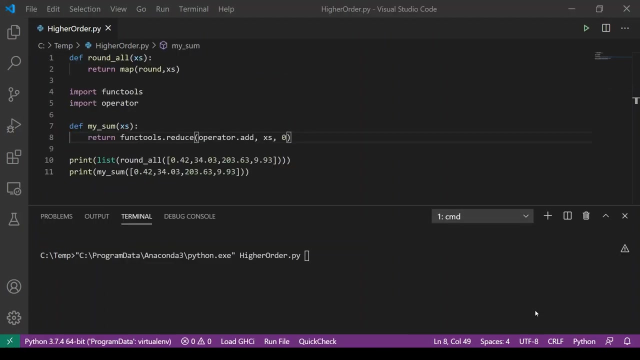 recursive approach and the higher order approach, And when I run this code down here, we'll see that we get the same result in each of those categories, whether using recursion or higher order functions, Though imperative programming languages are still much more popular than functional programming languages. 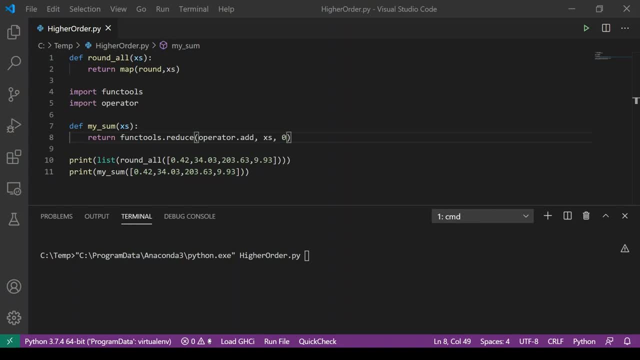 many features of functional programming languages have seeped into some of the most popular imperative programming languages. So I'm going to go ahead and show you some of these programming languages. For example, here is some Python code. Python has a map function And if you import the func tools module then you 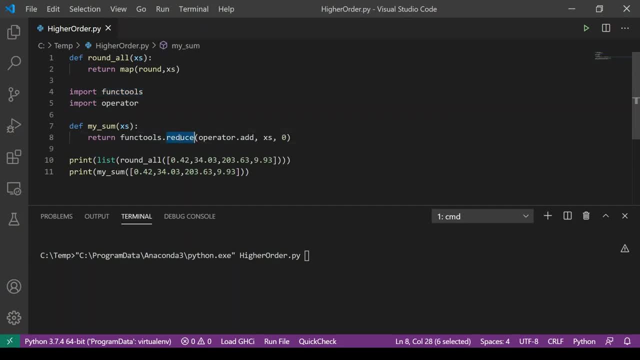 can also have access to a reduce function that is similar to the lisp reduce function and the Haskell fold functions. Note that I also import operator so that I can treat adding like a function, Because if I were to simply put a plus here, that would result in a syntax error since Python. 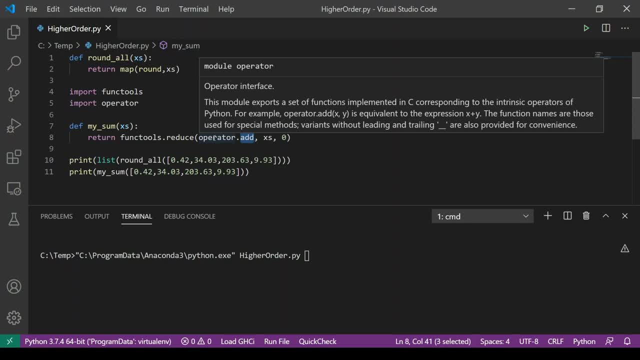 treats actual operators different from other function definitions. I test this code by printing the result of calling round all on this list and my sum on this list, And note that in the case of round all which uses the map function, I also convert the result to a list. 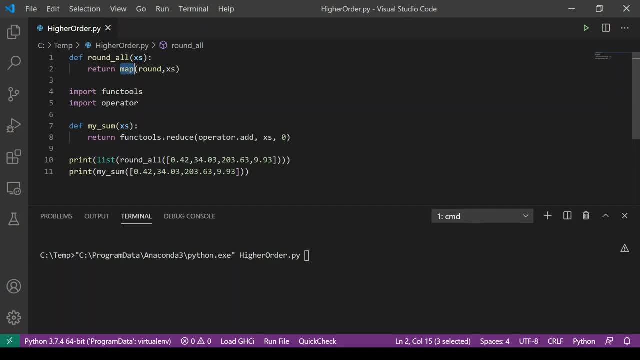 Python's map function returns a special type of map object, but if I want to simply see all the elements in order, then I can convert that to a list quite easily. Here is the result of running the code, showing you that it's straightforward to round those elements, or. 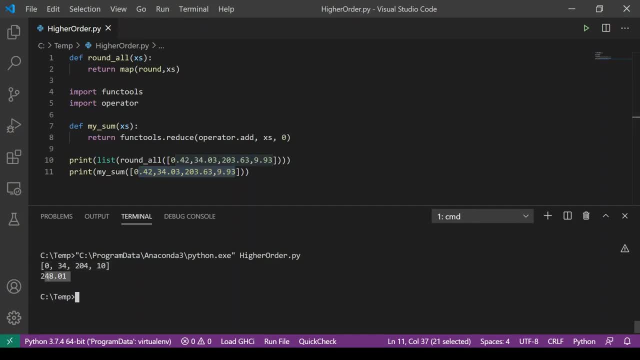 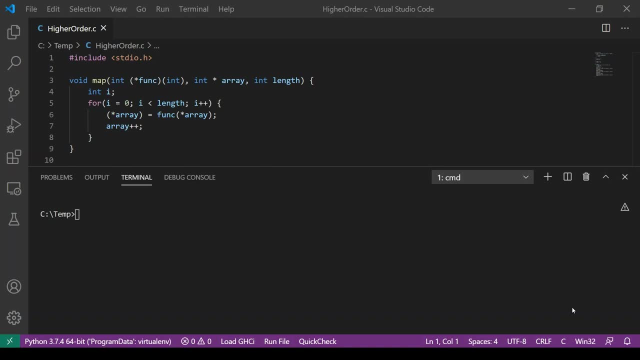 to add all of those up to get this result. Even an old language like C, which is very imperative, has support for a few elements of functional programming. In C one can define a pointer to a function And if you pass that pointer in as a parameter to another function, then you have. 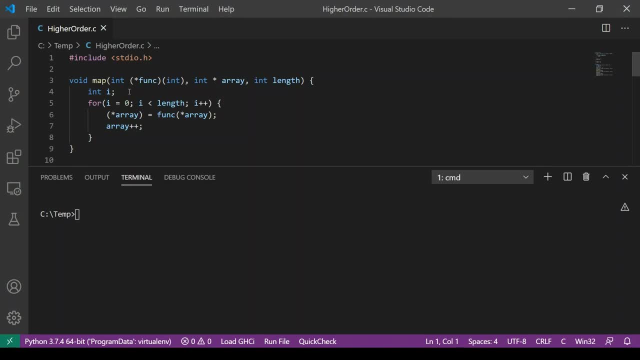 effectively passed a function as a parameter. That's a bit clunkier than how things are implemented in true functional programming languages, but powerful nonetheless. Here I'm defining my own map function. Now what I will do is take an array, although I'm actually using a pointer to the base element. 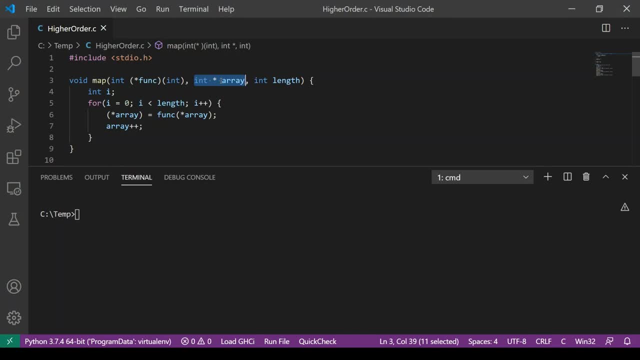 of the array, since this is a common way of passing arrays in C, And I also pass in the length of the array, since C arrays don't inherently know their own length. But what's interesting here from a functional programming perspective is this first parameter. This: 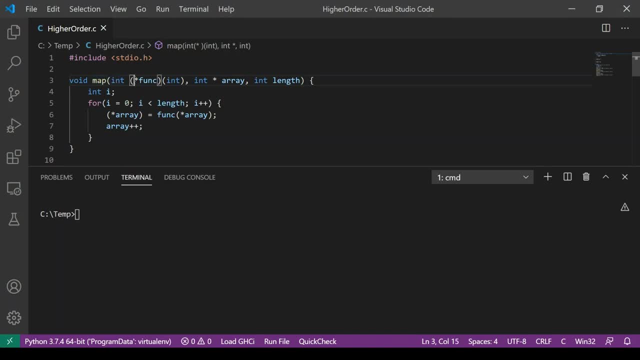 is a parameter whose type is a pointer to a function. the name of the parameter is func, and the type of the function is something that takes an integer parameter input and returns an integer, And so what I will do is repeatedly apply the function func to the input array, thus modifying that array to a function. 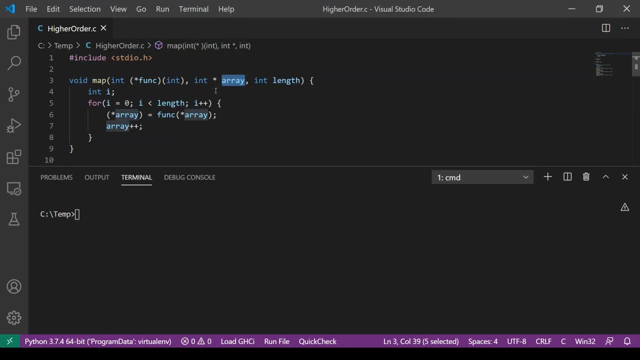 contain the result of repeatedly applying that function to each element. So I have a loop that goes through the length of the array By using this pointer syntax, pointer array. this indicates a particular element within the array, and so I am replacing that element in the array with the result of: 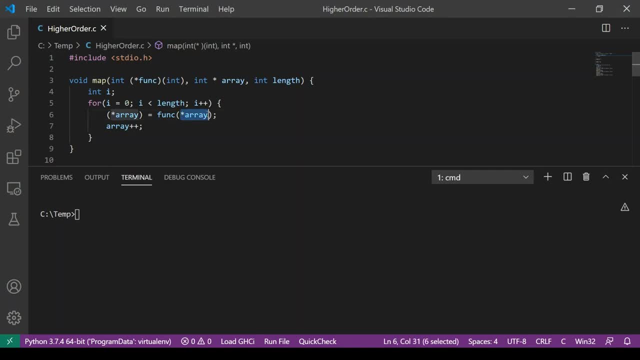 applying func to that same element and incrementing the array directly increases the offset where the pointer is in memory. so this is pointer arithmetic, which effectively moves to the next array element. Down here I've defined two simple functions whose type signature matches the type required as input here: An integer input. 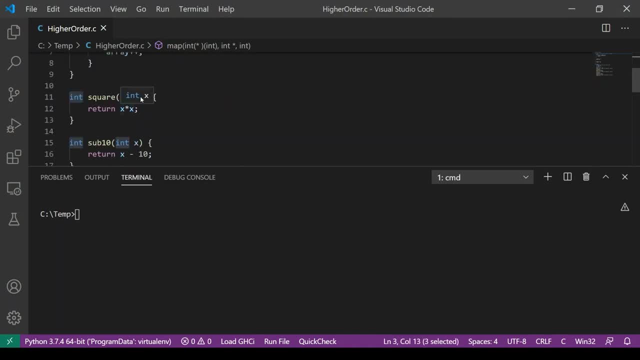 and an input sound code. Down here I've defined two simple functions whose type signature matches the type required as input here: an integer input and an input sound code. integer return value Square takes an integer input x and returns x times x Sub 10. takes an integer input x and returns x minus 10.. And down here in the